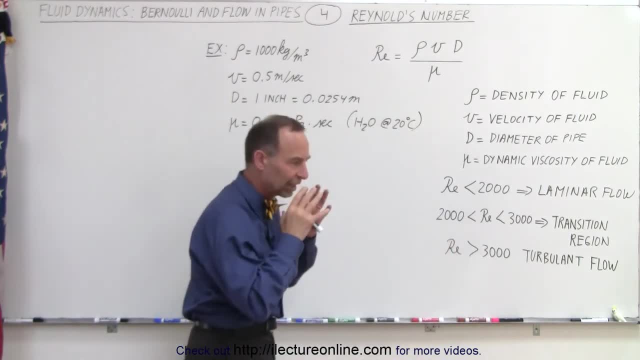 2,000, that means we're going to have laminar flow, which is steady flow through the pipe. If the number is between 2,000 and 3,000, we are what we call in the transition region, and then, if the number ends up being more than 3,000, we end up with turbulent flow. Now these 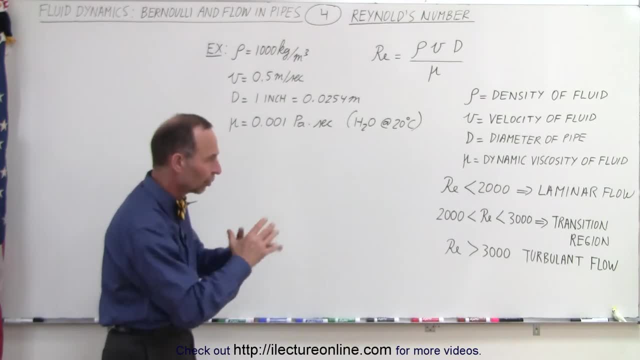 numbers are not exact and it depends from from fluid to fluid, but those are pretty good estimates. Now let's say we want to work on an example. Let's say we have water flowing through a pipe at 20 degrees centigrade. The denser water is a thousand. 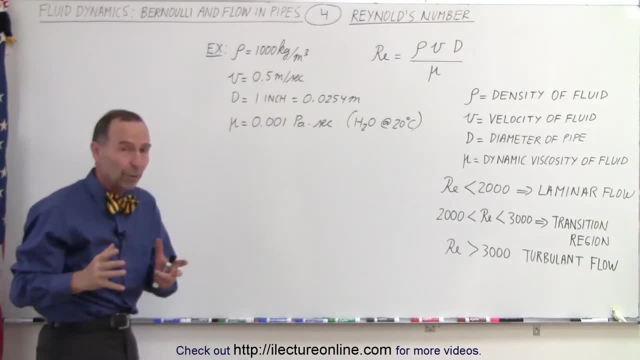 kilograms per cubic meter. Let's say the velocity is 0.5 meters per second and the diameter of the pipe is one inch, which is 0.0254 meters. and here mu for water at 20 degrees centigrade, the what we call dynamic viscosity of the fluid is 0.001, close enough pascals times seconds. So let's go. 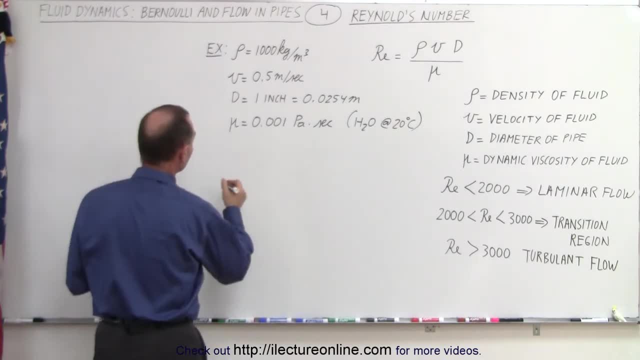 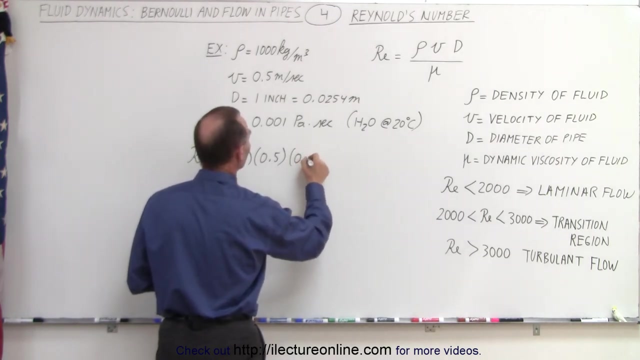 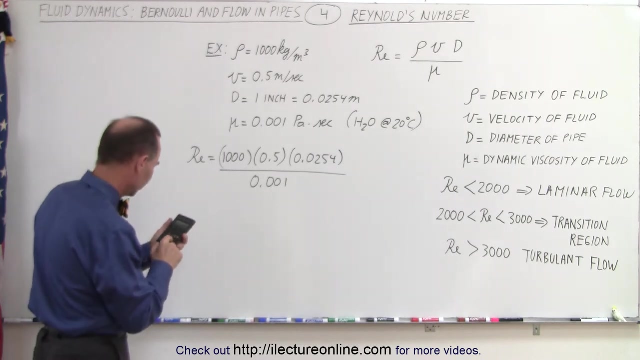 ahead and plug that in and see what we get for the Reynolds number. So the Reynolds number in this case would be equal to 1,000 times 0.5 times d, which is one inch, that would be 0.0254 all divided by mu, which is 0.001.. All right, let's see if that gives us a higher small Reynolds number. 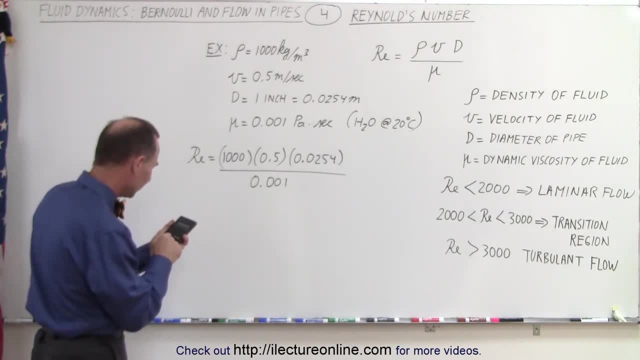 So we have 1,000 times 0.5 times 0.0254, divided by 0.001 equals, and we have a Reynolds number equal to 12,700.. So that is well over the limit of 3,000.. So you know that that's going to be a turbulent flow. 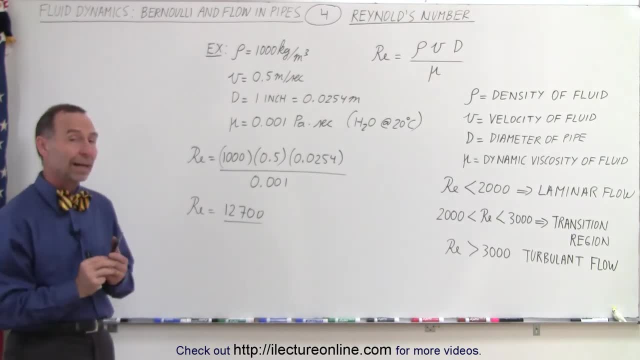 In other words, we're trying to push the water to the pipe- fairly small pipe and one inch diameter pipe- at too high a velocity and therefore that will not see it in a laminar fashion. it'll be a turbulent flow as we're pushing the fluid through and that's. how we determine the Reynolds number.